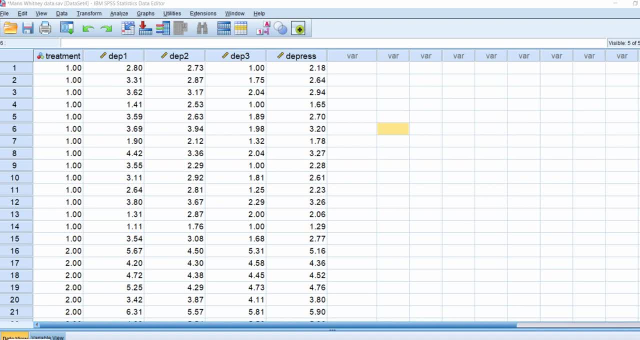 Hi everyone. In this video I am going to demonstrate the Mann-Whitney test using SPSS. The Mann-Whitney test can be utilized as a possible alternative to the standard parametric independent samples t-test when certain distributional assumptions are not met, such as the assumption that the data on your dependent variable are not normally distributed in your two groups. 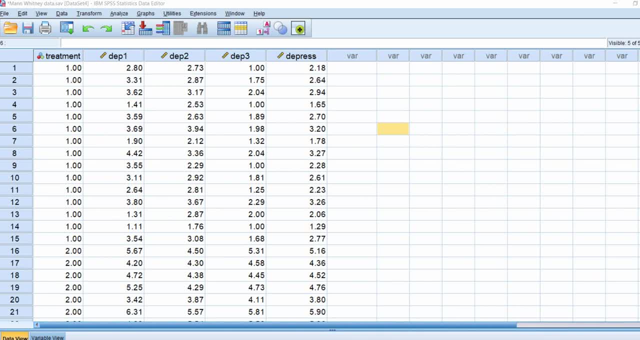 Now the independent samples t-test involves a comparison between your two groups with respect to their means. However, the Mann-Whitney test involves a comparison between two groups with respect to the mean ranks on the dependent variable. So to clarify what I mean by mean ranks, imagine that I have two groups of cases with scores on a dependent variable. Let's say it's a continuous dependent variable. 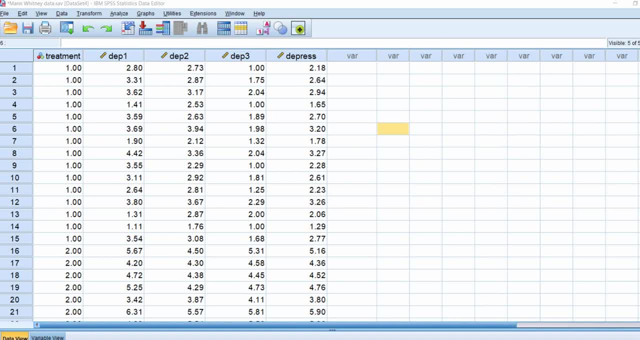 And I rank, order the scores. I rank the scores on the dependent variable from low to high, irrespective of group membership, and then compute the mean of those ranks for each group. So the Mann-Whitney test, then, would involve a comparison between the two groups with respect to those mean ranks. 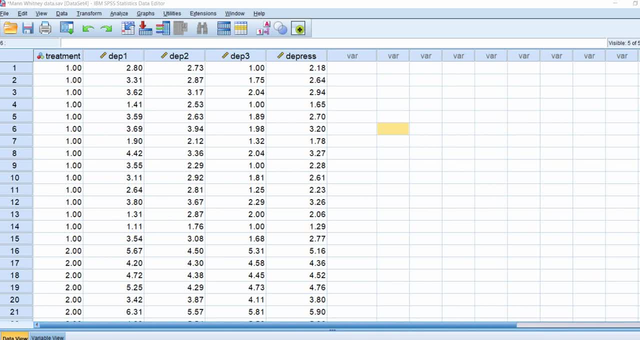 So, for our demonstration, we will be working with the data that you see on your screen and I am going to include a link underneath the video description for you to be able to go there and to download it, To download a copy of the data and to follow along. 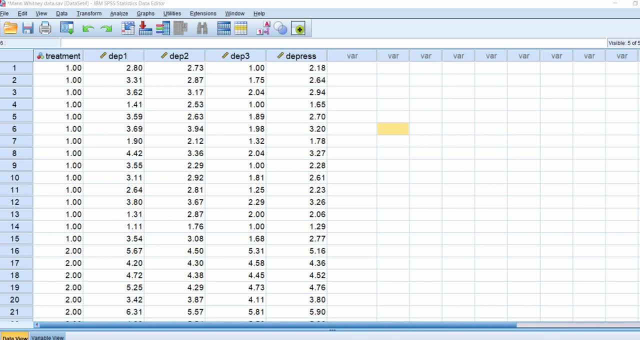 So the scenario that we will be posing in this case is one where I am a counseling researcher and I want to compare two treatment individuals in two treatment conditions on a measure of depression after a three week treatment period. So the independent variable treatment actually has two levels. 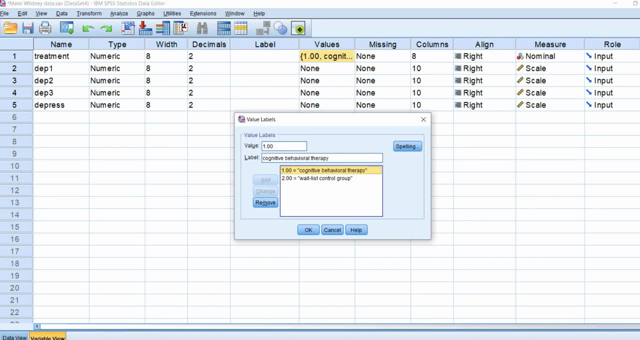 The level one is cognitive behavioral disorder. The level two is cognitive behavioral therapy, So individuals who will be randomly assigned to that treatment condition. And then level two is a wait list control group. So those individuals for a three week period are not going to receive the treatment, although we would ideally have them receiving the treatment afterwards. 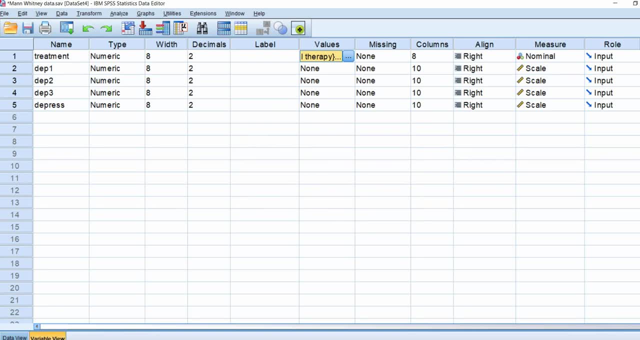 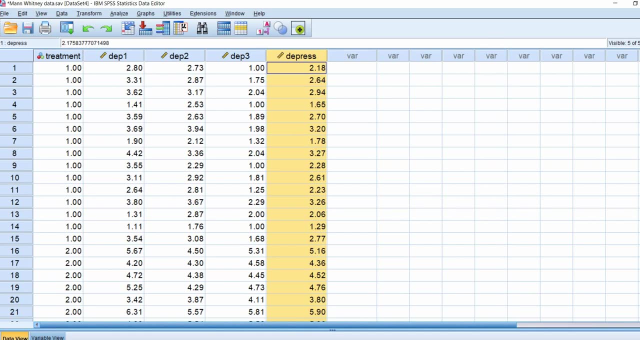 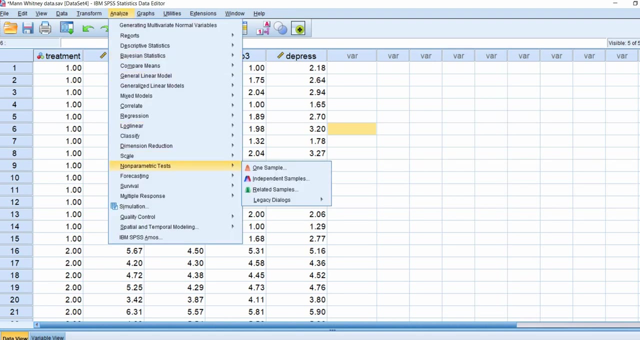 So we will click on OK. And our dependent variable is depression. So this is measured as a continuous variable. And to carry out our analysis, what we will do is to go to analyze, Go to nonparametric tests and then to independent samples. 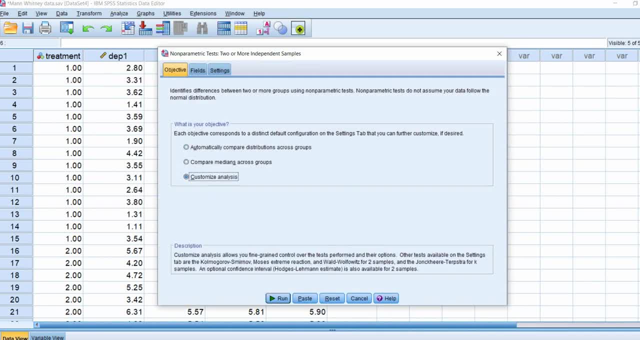 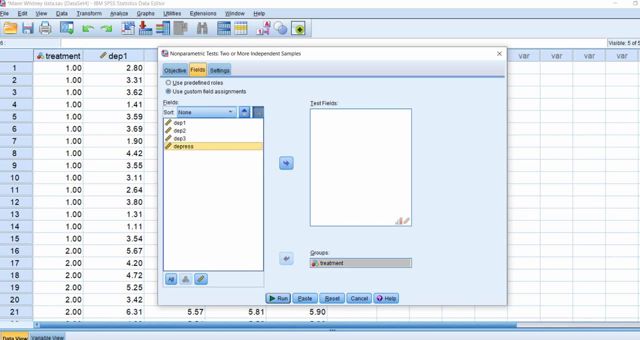 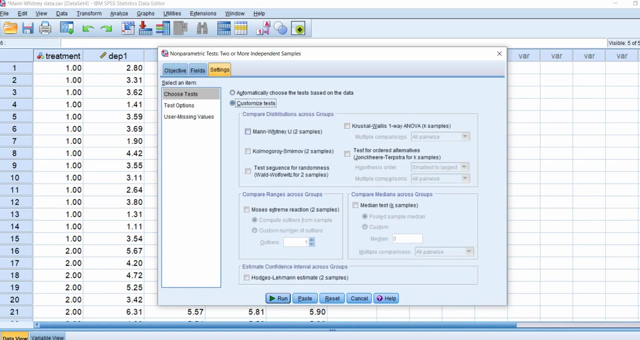 Under the objective tab we will click on customize analysis and then move to the fields tab. Move our independent variable down to the groups box and then our dependent variable over to the test fields box And then we will click on settings. Go to customize tests. 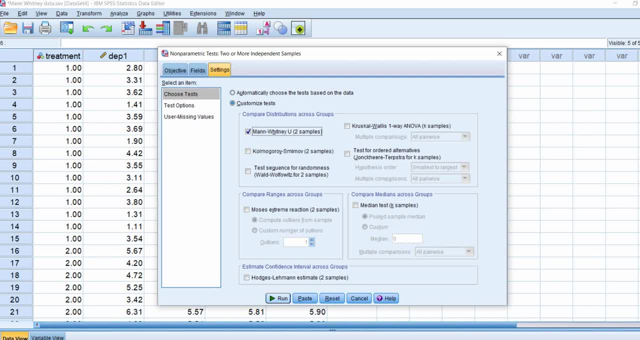 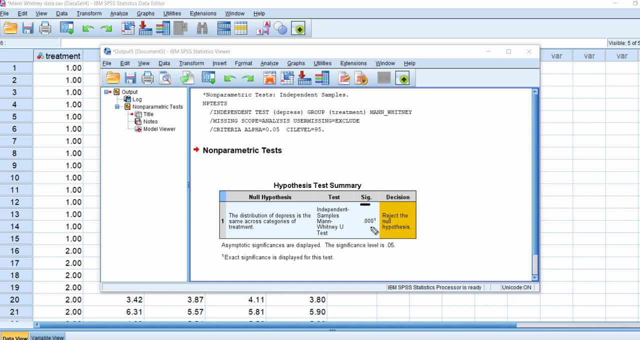 And then we will click on man Whitney to samples. So then we will click on run And we get our output. So right here you can see that we have the significance level given. So our p value: It says .000.. But we would report this as p less than .001.. 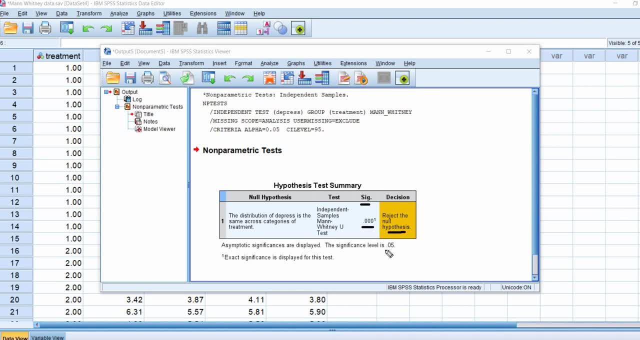 And they also give you a decision right here where there is a comparison of this p value against the alpha level of .001.. So next, what we will do is double click in this box And you will see that the pane on the right gives us some more information. 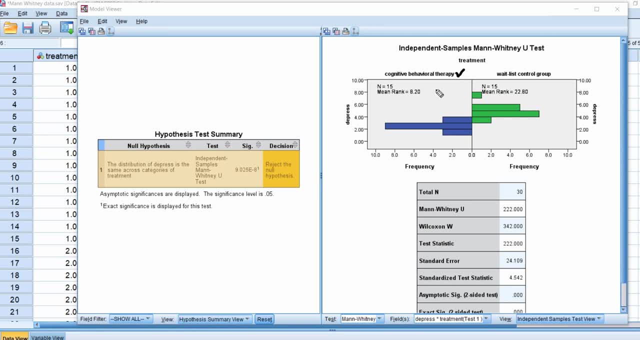 So you will notice that for the cognitive behavioral group, the mean rank for the depression scores is 8.2.. Whereas for the weightless control group, the mean rank is 22.8.. So what that is telling me, then, is that the scores in the weightless control group tend to be higher. 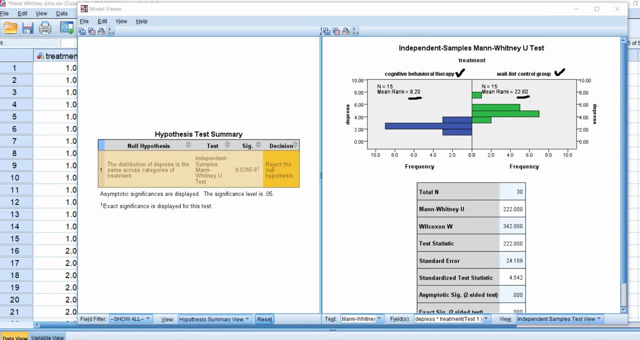 Than those in the cognitive behavioral group. Okay, so next you can see that we have essentially our man Whitney test statistic. that is given right here, As well as the p value. asymptotic significance for a two sided test Where you have p would be presented as less than .001.. 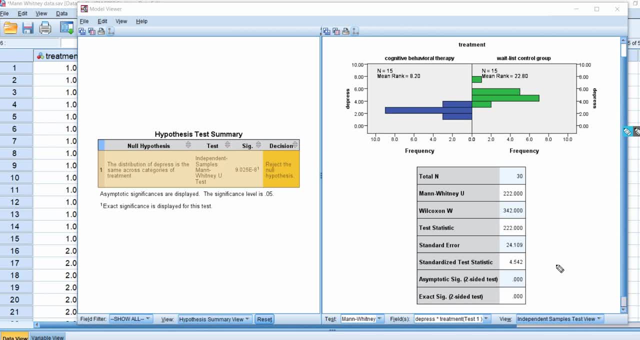 You will notice too that if we scroll down here A little bit further, we have an exact test that is given. There is our p value, And this is actually the same value that we had seen over here, Where they said the exact significance is given. 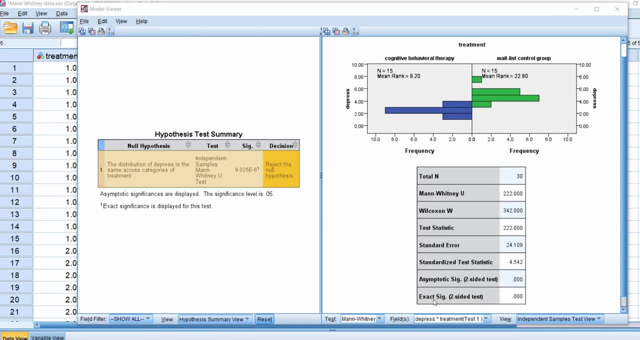 And generally, you would want to choose the exact significance in cases where you have smaller sample size that you are working with Now. looking at this table too, You will notice that there is a Wilcoxon W that is referred to here, Basically the Wilcoxon W. 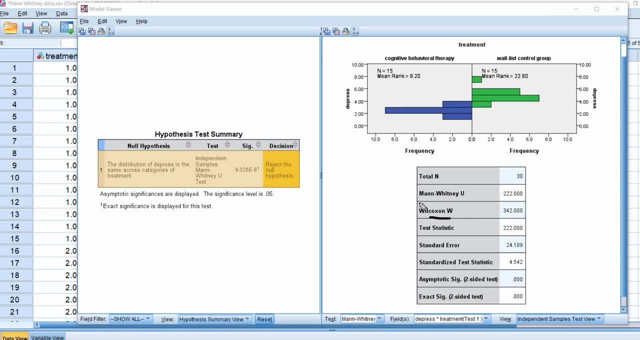 Is essentially going to give you the same results as the man Whitney. They are fundamentally the same thing. And then down here, this is a Z value And you can still utilize the significance levels that are associated with that test. So if you wanted to present a Z value instead of the man Whitney, U. 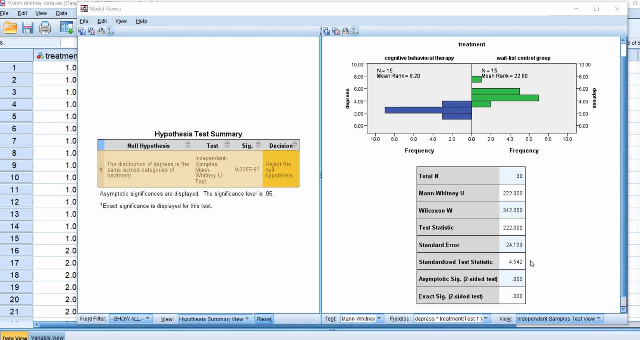 You could certainly do that using that standardized test statistic that is given below. Okay, so that pretty well concludes this video Demonstration, and I appreciate you watching. 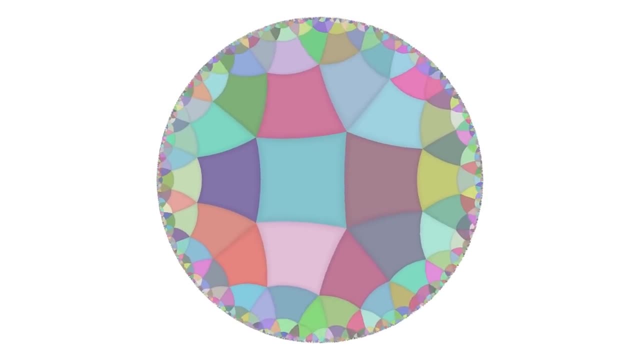 In my Hyperbolica devlogs I mentioned you can build a model of hyperbolic geometry using crochet, but I never learned how to do it myself Until now. It's actually really easy and I'll show you how to do it in this video. But there's an even more fundamental connection. 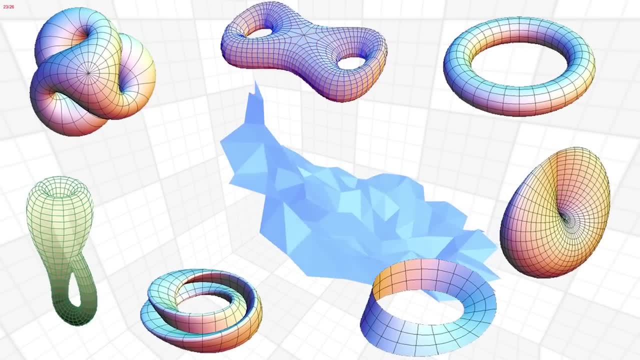 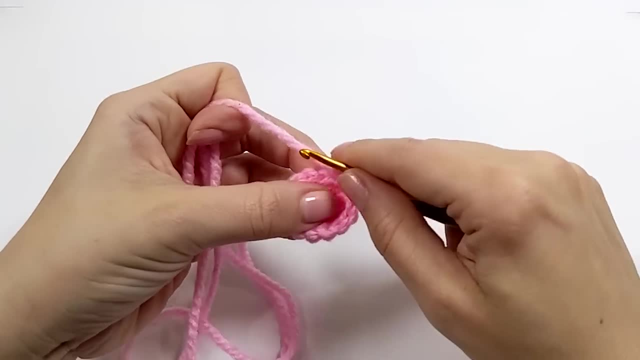 between crochet and topology. so let me show you why it's so cool from a programming and mathematics perspective. Normally, crochet adds to a piece one stitch at a time, as you kind of spiral around, But what you're really doing is building a mesh. 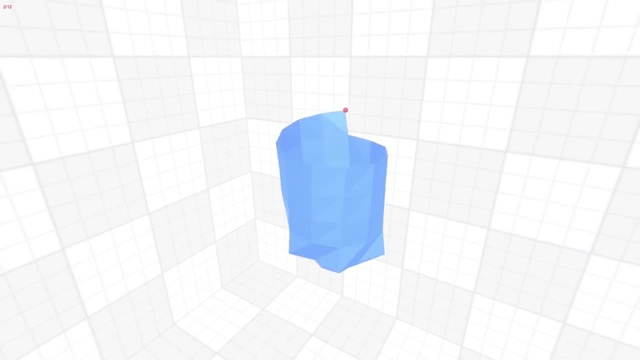 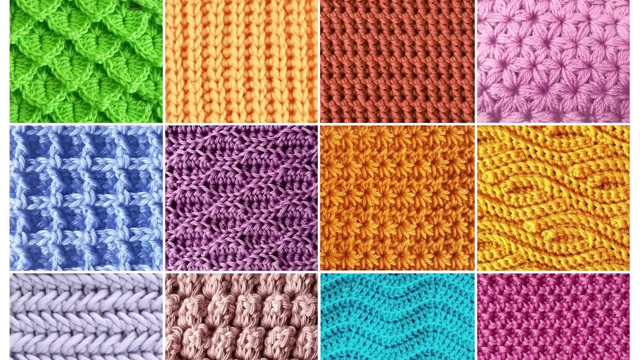 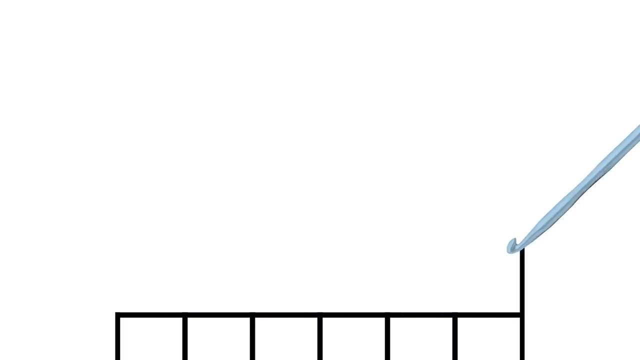 just like you would in something like Blender. In fact, I built this crochet simulator to show how that works. To be clear, there's like a million different kinds of fancy crochet stitches, but ignoring aesthetics, there's really only three that you need. Let's unwrap a cross section. 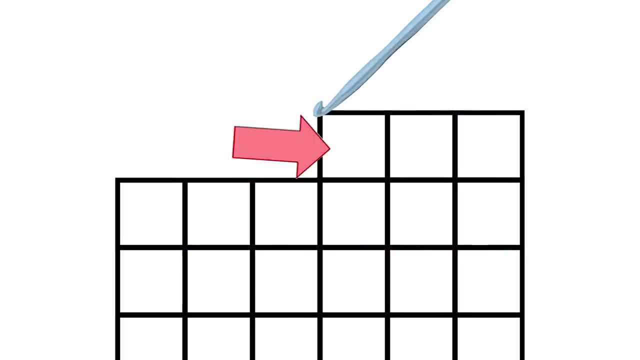 so you can see what I mean. These square stitches are the simplest kind, called single crochet. so let's say your hook is over here and you add a single crochet. The previous row is now connected to the new one and once you spiral around to the next row you can hook onto it again.